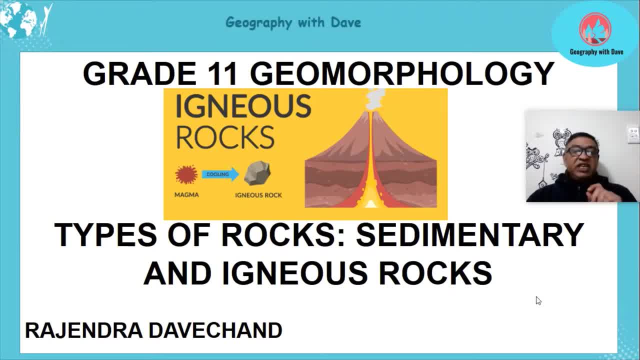 revise over sedimentary and igneous rocks before we look at the horizontal strata, the inclined strata and massive igneous rock strata. Alright, because we need to have the background information in order to understand those processes. So this is basically a revision. 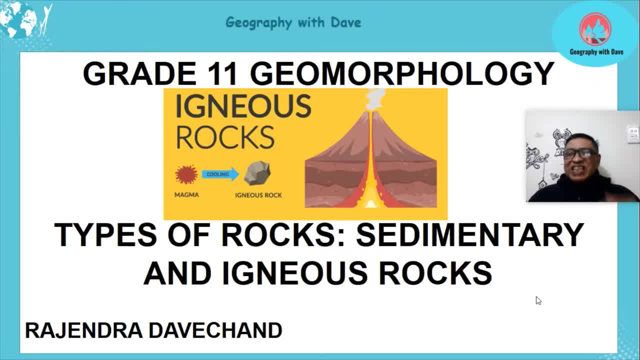 of your grade 10 work. I've also included things like significance. Okay, so we're going to look at the structure and the characteristics of these two rocks, or types of rocks. that's going to assist us with those other sections. Okay, So many of you know it already. Alright, because you've learned your grade 10 geography. 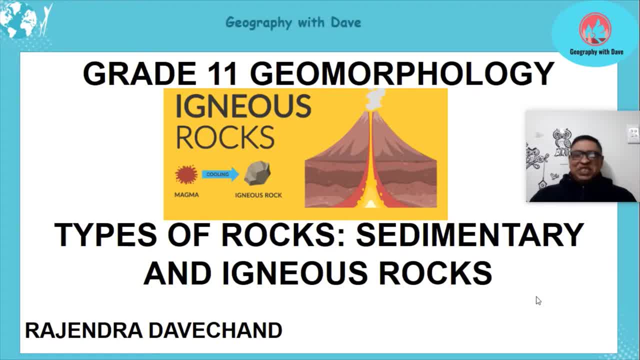 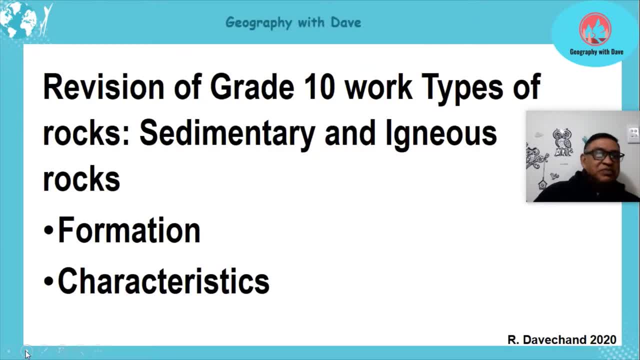 well, Okay, so it's just a matter of revision. Okay, so let's get going with this, All right. Now in this section, we're going to look at both rocks again. Let me get my highlighter. All right, we're going to look at the both types of rock: sedimentary and igneous rock. 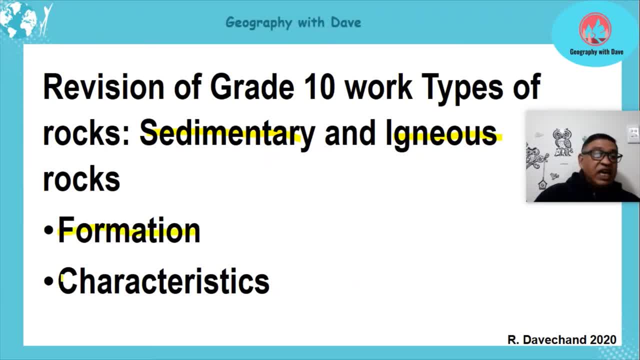 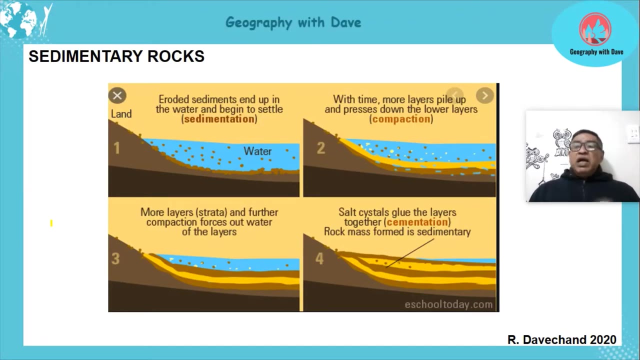 And we're going to look at their formation and characteristics. Okay, remember, this is necessary. Okay, for understanding horizontal inclined and massive igneous rocks. Okay, so let's start. We've done it in grade 10.. We know how sedimentary rocks form. First, 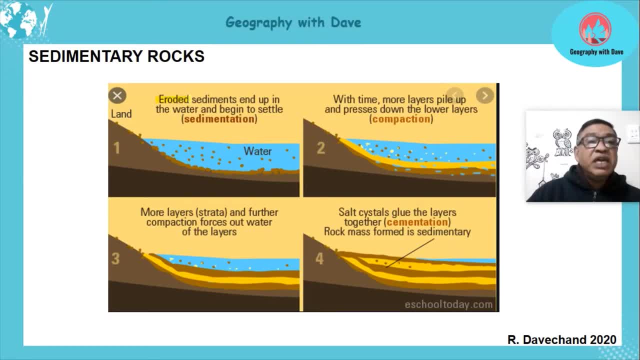 thing is about erosion, Okay, which occurs, Okay, And what actually happens? the sediments end up in water and they began to settle. That's your sedimentation And of course you must remember the erosion is a continuous process. So what happens next? Wood time, more layers pile up. So you had 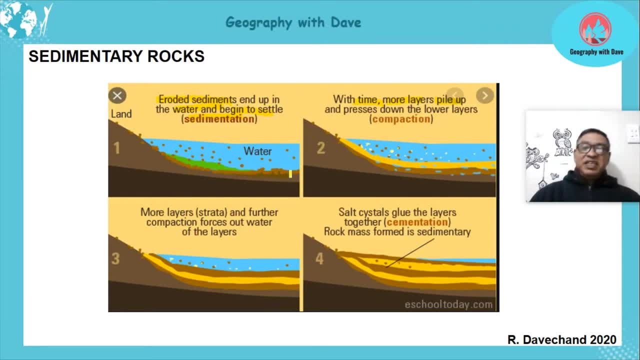 the first layer. Can you see it? But as more erosion occurs and sediments get deposited, another layer forms- Can you see it? Okay, and they press down on the lower layers. So what happens is, when this layer presses down on that layer, it becomes more compact, solid, more compact. 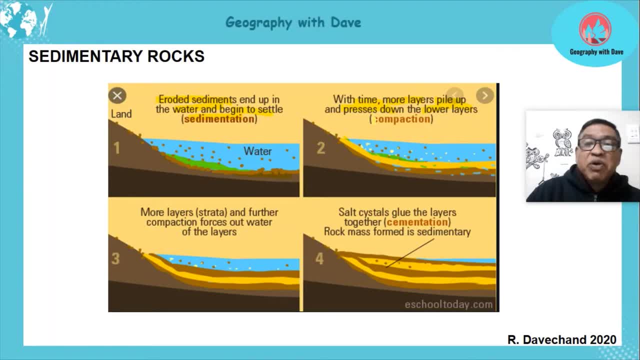 All right, And that's what we call the process of compaction. Same thing you did in grade 10, eh, And then more layers and further compaction happens which forces out the water of the layers. All right, So as more compact, more compact, whatever humidity or 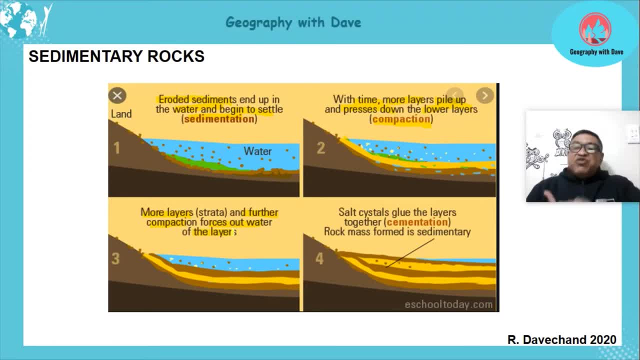 water is in the layers now actually is forced out. It becomes more compact and solid. Right, Soled crystals glue the layers together. All right, The crystals that's found there actually solidify and glue the layers together So they become one rock with many layers, Right. 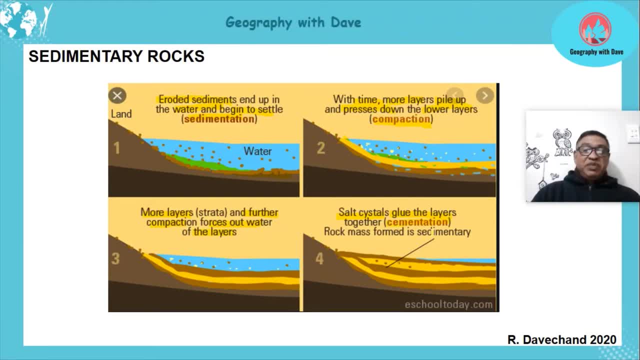 So that's known as cementation And eventually your sedimentary rock is formed. You just get it. You don't get all loose layers. There's compact cementation happening with the soil crystals that's in there and it solidifies it and it becomes one rock. That's your sedimentary. 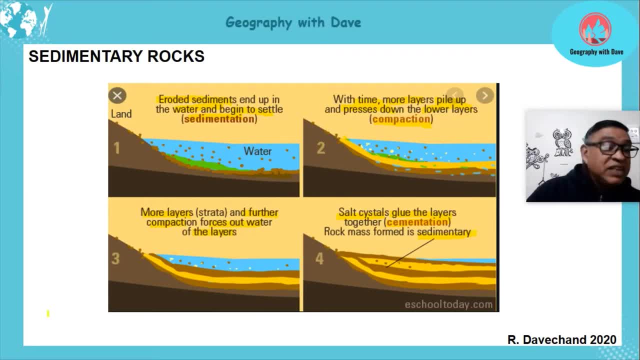 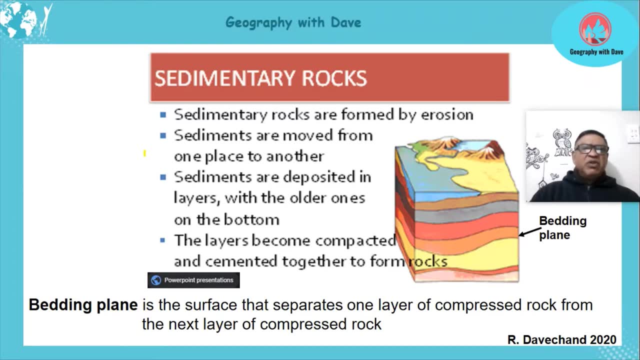 rock. Okay, As you've done last year, as I mentioned. Okay Now. so let's look at the overall aspects of it. All right, It's formed by erosion. We know I'm going to keep repeating it in my slides, So we'll reinforce the idea. Okay, And I'm going to go back. I've always done. 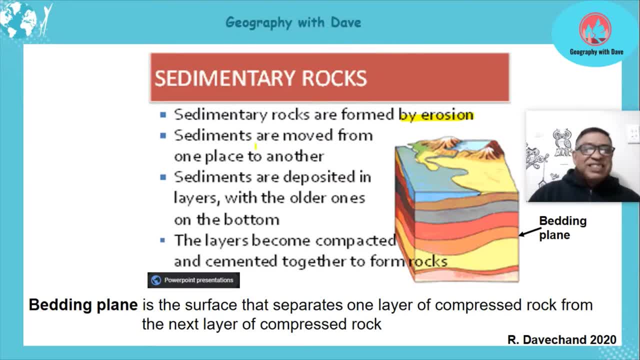 this when I move my fingers too fast, Okay, From erosion. And then sediments are moved from one place to another. Remember, erosion will take it from the land and deposited into the water. All right. Sediments are deposited in layers, Okay, Remember, we said that the 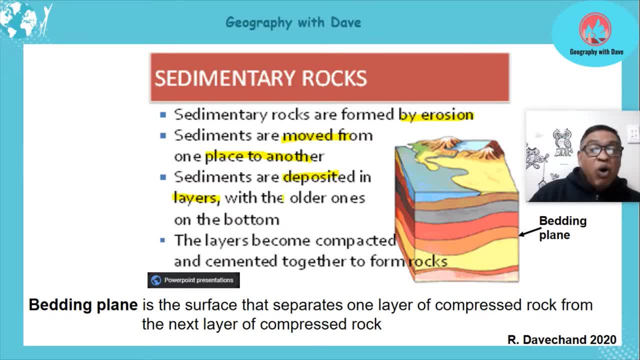 first layer, further erosion, another layer with the older ones at the bottom, All right. And as they become compacted and cemented together, Okay, Okay, They form the rocks, which is your sedimentary rocks. All right, Now, in between these layers, 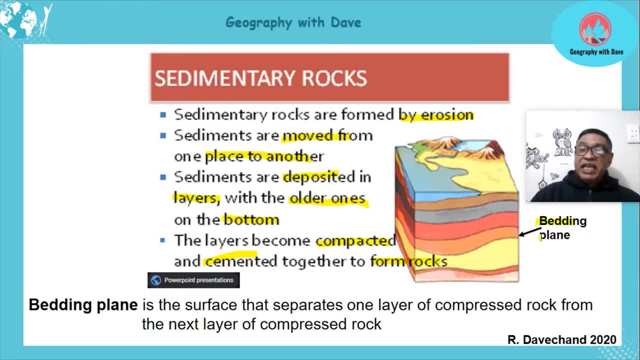 of rock. there is a bedding plane. All right, What is the bedding plane? It is the surface that separates one layer of compressed rock from the next layer of compressed rock. Okay, That's why you can see, it is found between the layers, all right, of the rocks. That's. 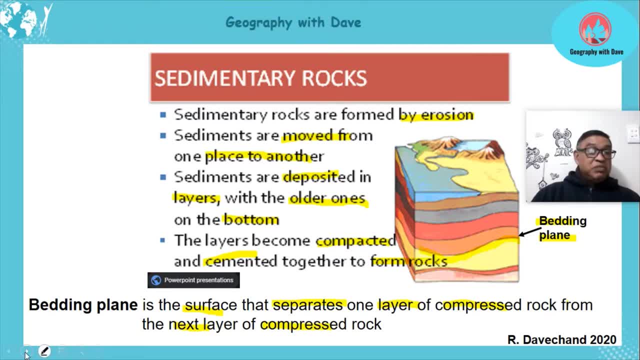 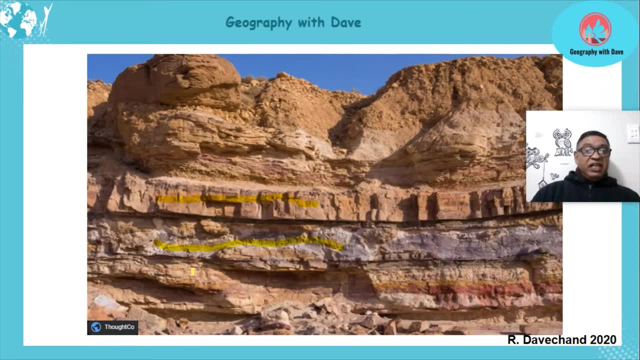 your bedding plane, Something for you to know also, which is important. All right, You can see a picture here. Can you see the layers? There's another layer, There's another layer, And this is your sedimentary rocks. And in between the sedimentary rocks, there is your. 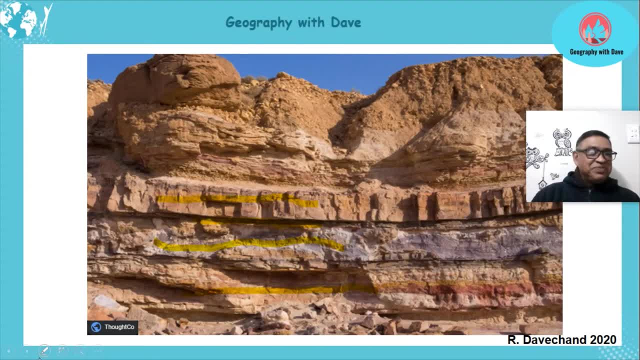 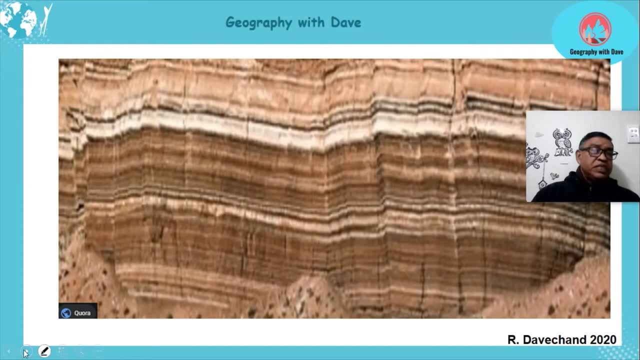 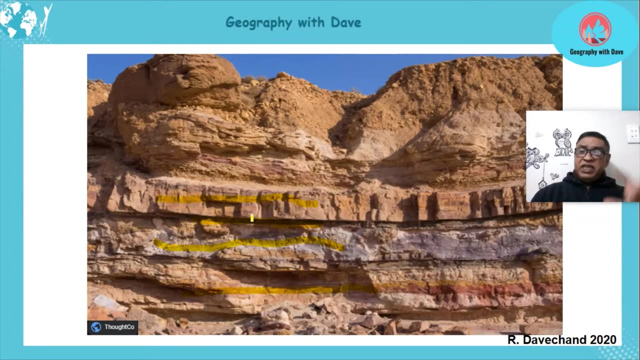 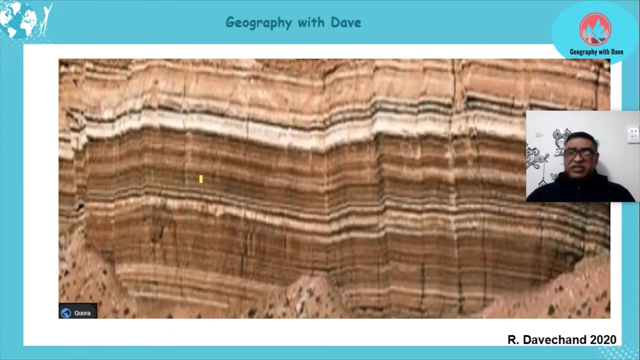 bedding plane. okay, right now i'm showing you another picture, because what i want to show you here is that, yeah, there's larger layers. okay, right, there's thicker layers and here there's thinner layers, so we can get layers that vary in size. all right, sometimes it's harder to see the layers. 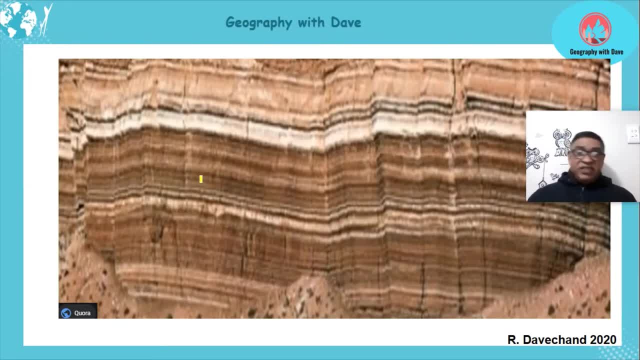 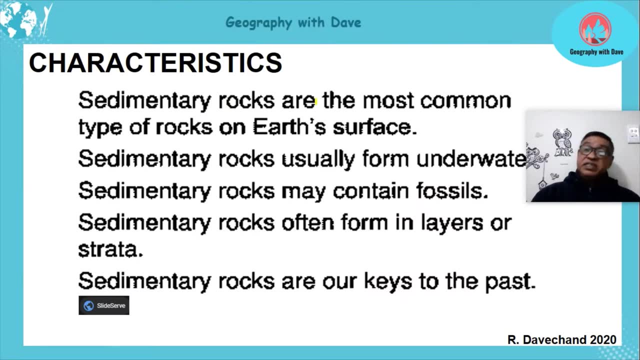 sometimes it's easier when they begin, so they vary in size. just remember that all right. now again some other characteristics and some i'm repeating. they are the most common rocks that are found. okay, next one: they usually form underwater. let me move my face a bit underwater. remember they usually form- not always, but they usually form. and 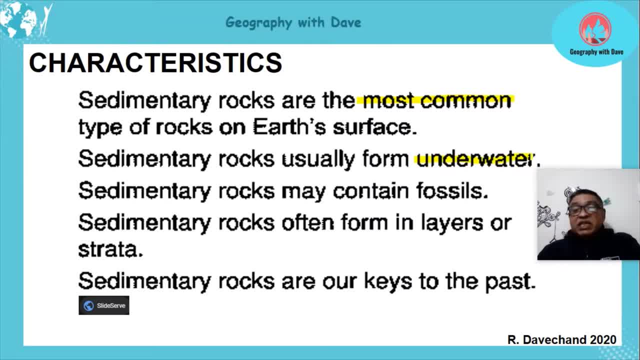 that's the main characteristic. all right, as sediments get deposited, a layer forms in the water and the next layer forms in the water. all right, they may contain fossils. all right, as the sediments form, uh, animals die, plants and they all get part of that rock which becomes. 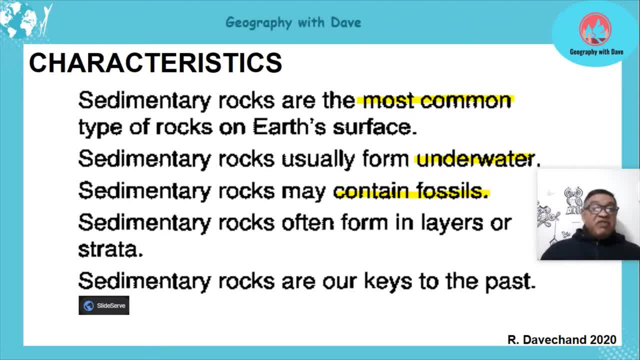 compressed and as you dig up rocks like this, you may find fossils. and another thing here is that the hands are very fidgety today because i have to apologize for that, and the sediments are very fidgety today because getting small and big- right, i do apologize for that- and the sediments 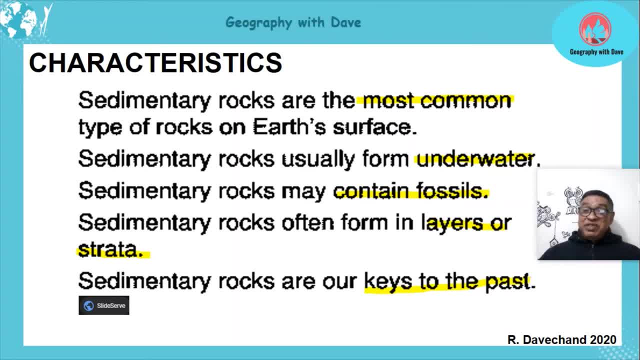 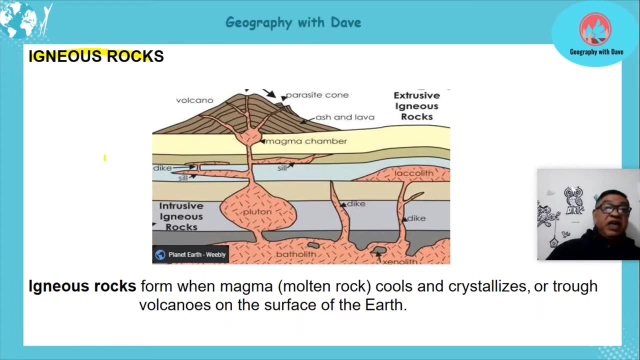 are key to the past. okay, because you can find fossils. it tells us about the past. you must know ever fossils that were there in the past. we can learn more about it. just giving you an example. all right, let's go to the next slide: igneous rocks. now their formation is different. 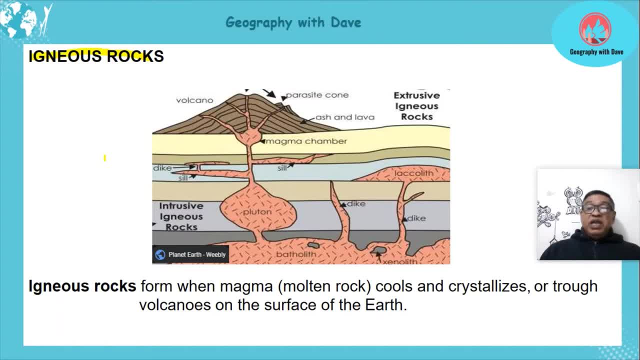 when you do volcanism or something so volcanism, you will learn that magma is found below the surface of the earth and as it comes to the surface, it's known as lava. all right, as you've done in the past, you've learned this okay, but you must know that as this magma moves, it also 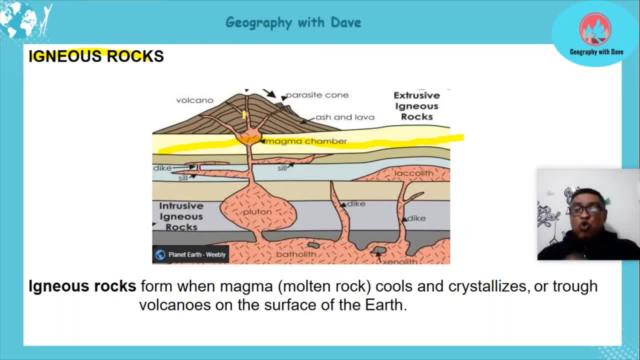 receives creatures, temperatures where it will cool, okay, it will cool down and it will solidify and therefore various features will form within the ground. but when that solidifies, it becomes igneous rock, all right. so obviously around it, can you see all the layers, all the layers around it? that is your sedimentary rock. 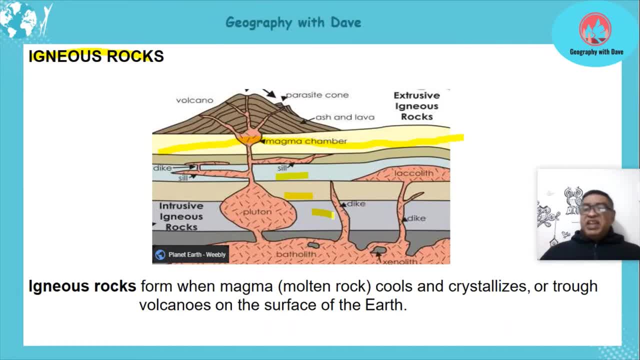 which you'll have last year, is considered to be softer. it'll vary in resistance. obviously, all right, uh, but it's considered softening. as this gets eroded, these solidified magma here gets exposed to the surface as igneous rocks. okay, that's one way in which igneous rocks 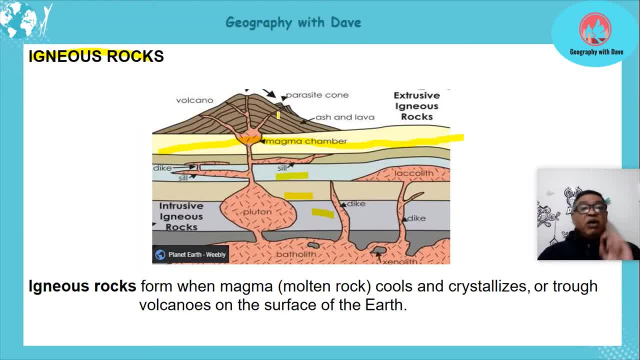 will form. okay, the cooling of the magma, all right. now let's look at another thing: the volcanoes. when they erupt. can you see this volcano erupting here? it's coming out in all directions and as it reaches the surface it will cool also, and as it 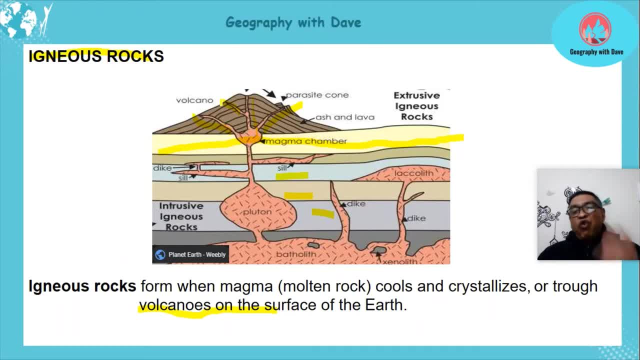 cools, it solidifies and will form igneous rocks. so if you look at it, it can be formed below the surface as magma cools and it's been formed above the surface as lava cools when it comes through a volcano. all right. so it cools and crystallizes- all right, crystallizes lots of crystalline texture. 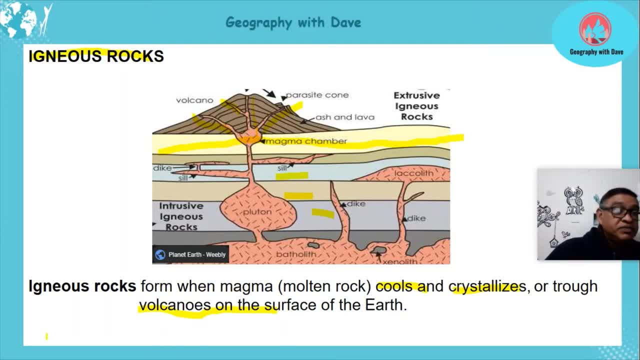 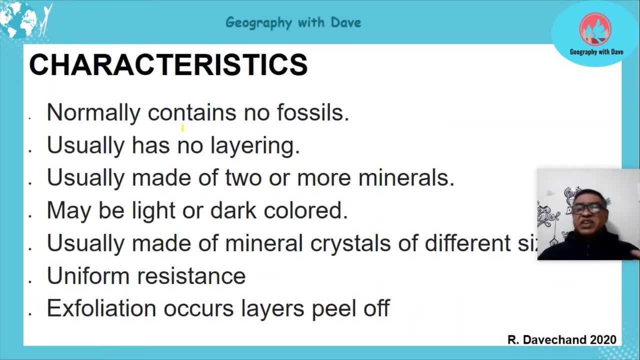 in the igneous rock. all right, and i'm going to the next slide. so some characteristics of this rock. all right, one of them, you would have seen, is that it has no fossils. no fossils, okay, in this rock it's crystals, minerals etc. that solidify, but fossils are not found in. 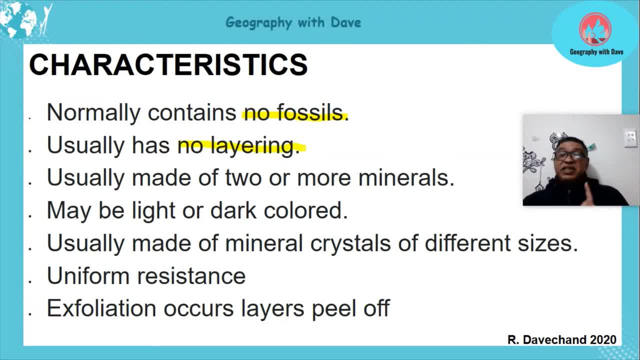 it has no layering, no layers. you remember, sedimentary rocks have different layers. igneous rocks have no layers. all right, usually made up of two or more minerals that are found in this type of rock- okay, good, solid minerals. it may vary in color also. it may be light or dark colored. 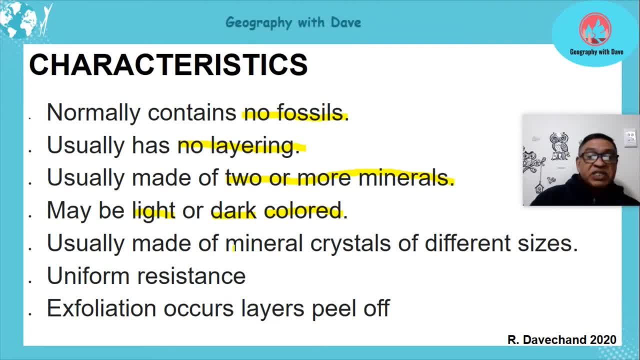 all right, usually made up of mineral crystals of different sizes- okay, different sizes of mineral crystals, as you've learned last year. okay, and then it has uniform resistance. if it's, it's a hard rock and it's a hard rock throughout the rock. it's just a hard rock. 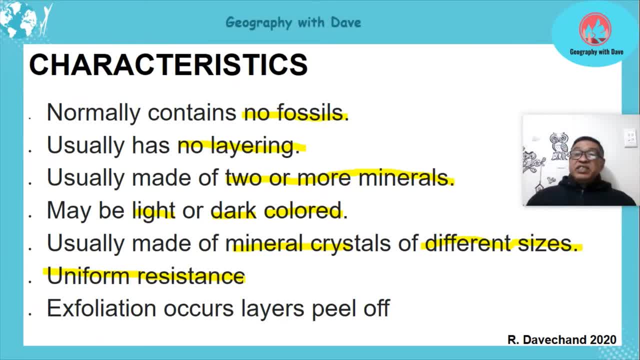 okay, and this one also has uniform resistance. if it's, it's a hard rock and it's a hard rock throughout. you don't get soft hard, soft, hard. the resistance is the same across the rock, whereas with sedimentary rocks the resistance can vary from hard to soft. not soft, yet it stays the same. all right, you have. 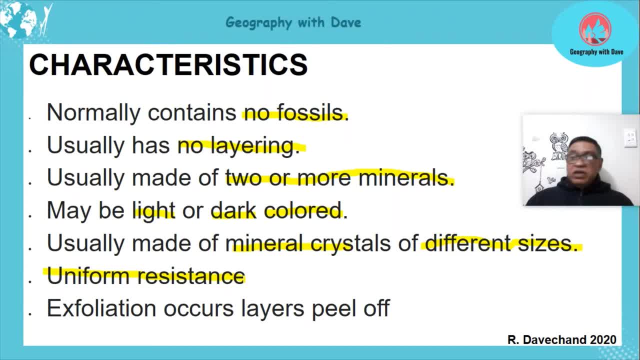 same hardness across the rock. is that clear learners? then it also experiences exfoliation- all right. when it's released, all right. you find various processes involved: weathering, etc. of course, we're not going to go into detail on this now, all right, but we're going to significant fact. 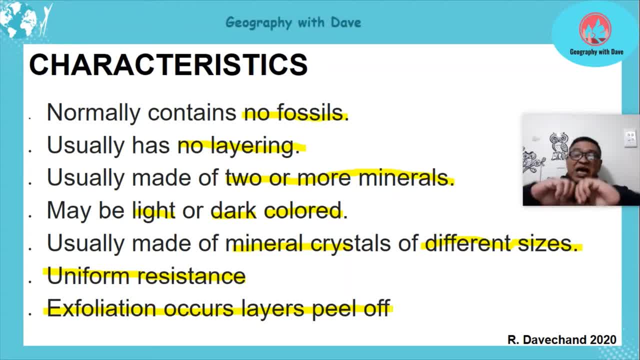 of exfoliation happening, where layers actually peel off from there. we always use the onion when we teach this, but please don't write the onion in your exams, all right? well, it has different layers just peeling off, like how you peel off an onion due to exfoliation. we're more focusing on what you need to know. 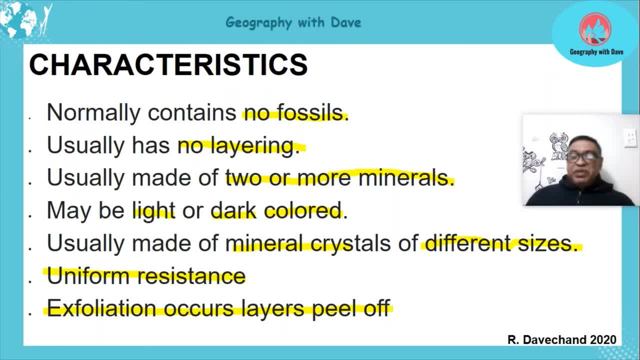 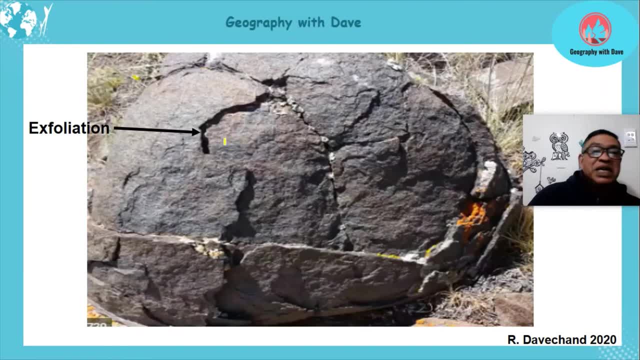 for grade 11.. of course, you went into more depth in grade 10. okay, right, let's go on. can you see the exfoliation happening here, where layers are coming out of peeling off? pieces of the rock are peeling off. i shouldn't be using the word layers, they're peeling off. 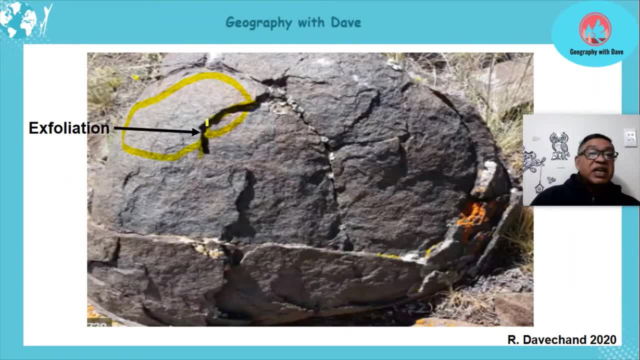 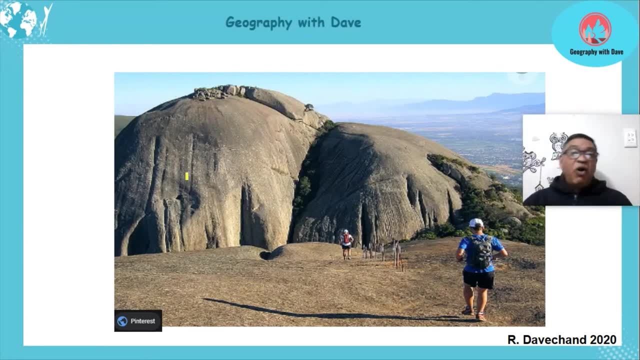 can you see? it's a solid piece of rock but layers peeling off down there right. look at this. this is your pearl rock. all right, huge. it most probably is a better. that came through. you understand that. let this come through and say: most use most brny. it is a battle it that comes. 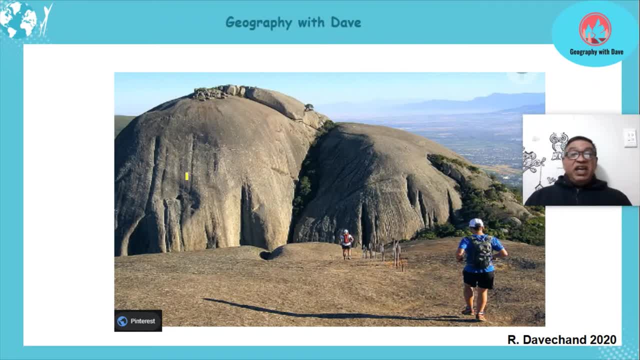 through. you understand, in this mass of rock here that has been exposed, the softer rock around it, the- it is marcuto rock. you understand, you don't have any evident rock. you have all the- yeah, interim rock that has been exposed, the softer rock around it, and the soft rock always comes out of it. indeed, it's easier than i out. it goes on the apparent. all right, i understand, you understand, if it's a. 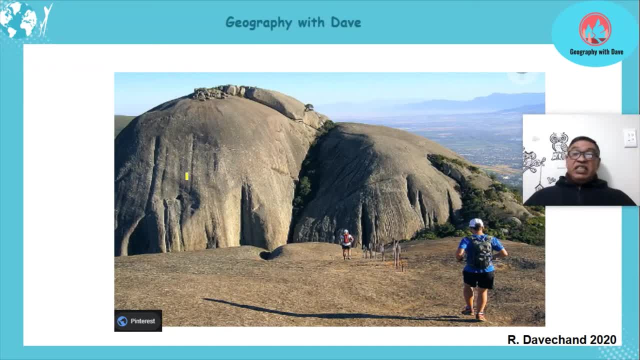 has been eroded and now we find this being exposed as a huge dome. later on you'll be coming across these features. you can see the resistance is the same across the rock. no layers, nothing of that sort. okay, it's just a solid system piece of rock. all right, that is your igneous rock, right some? 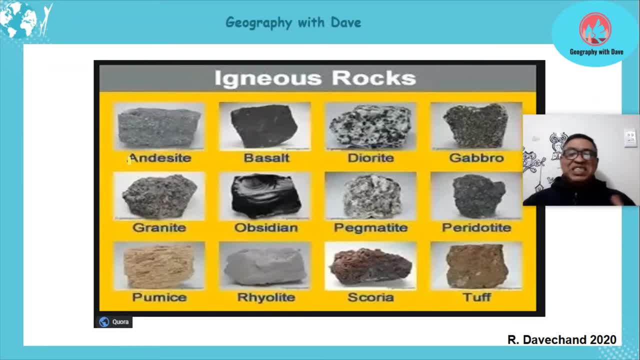 examples: yeah, uh, learners, you don't need to get into detail about this, i just thought out of interest. maybe you can identify these rocks when you see them right? different names: basil, diorite, gabbro, granite. uh, you don't need to worry. all right, you're not the geologist, okay. 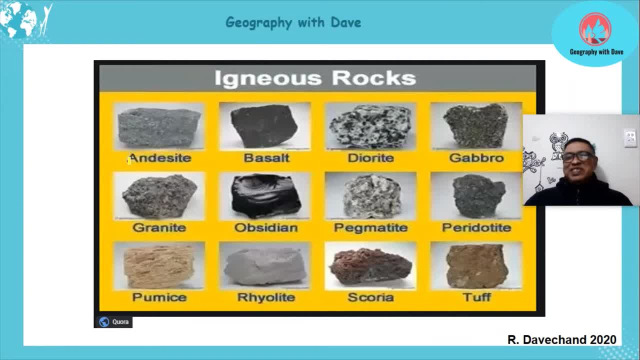 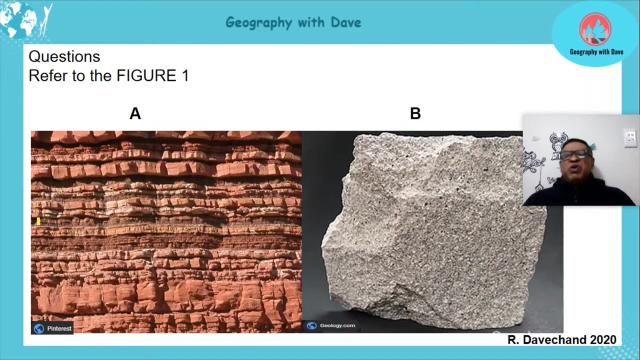 so I also have my own little rock collection that I go around. I don't damage the environment, you understand, but if you get a piece, it's fine. okay, right, those are your rocks. okay, now, i just gave you a little exercise on this, okay, uh, I also have my own little rock collection called the rock collection. 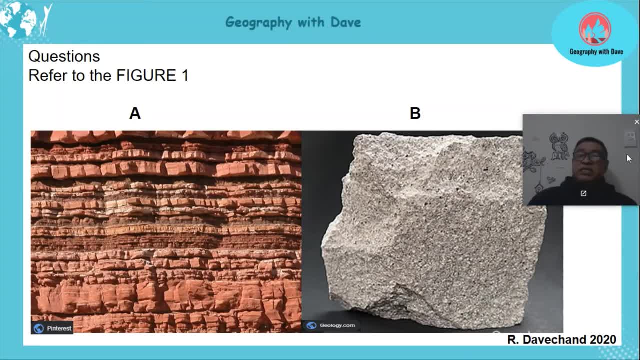 figure that i have in front of me and if you look at it right, there's two rocks here. it says: refer to figure one which has a and b. okay, and of course it's showing us two different types of rocks here. one: we clearly see the layers, can you see it? with its bedding planes in between. 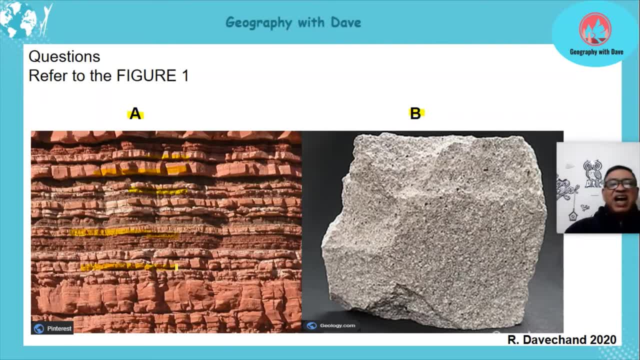 so we know that this is our sedimentary rock, okay, uh, this we see solid. we don't see any layers, can you see? in fact, i'm being naughty. i'm creating little layers there now, which i shouldn't. all right. so this is our igneous rock, remember, there is another type metamorphic. 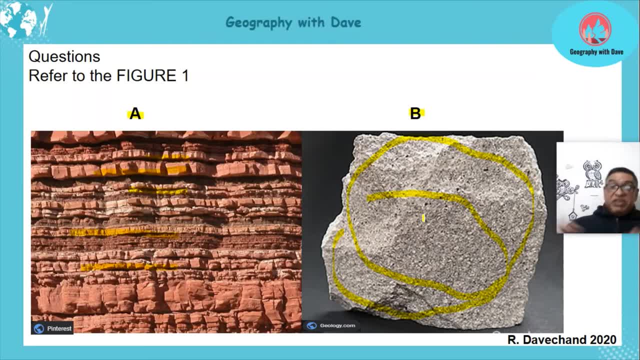 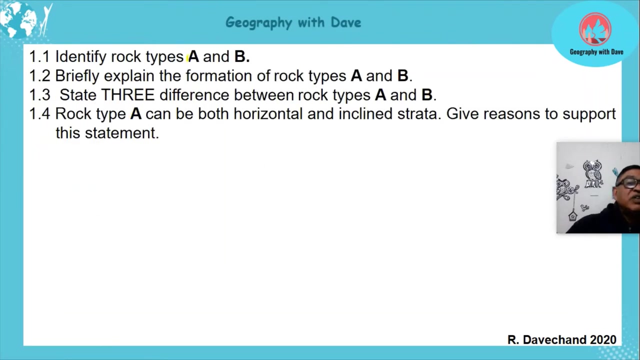 but that's not relevant to us in grade 11.. all right, we just focus on these two types. so we picked it up already. all the information that we learned so far will come through some simple questions or just to get your mind thinking. it's always important to have it all right and let's look at the questions. identify rock types a. 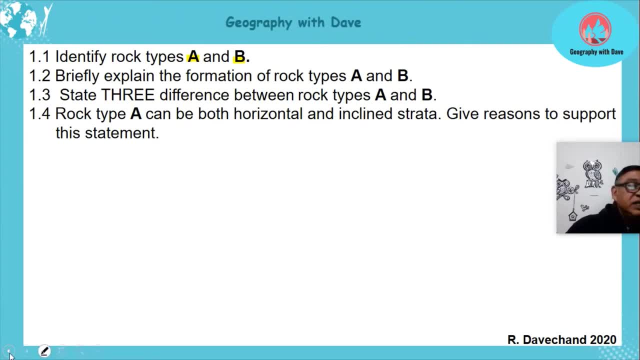 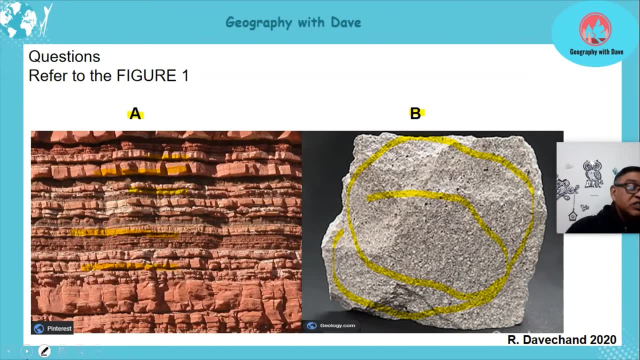 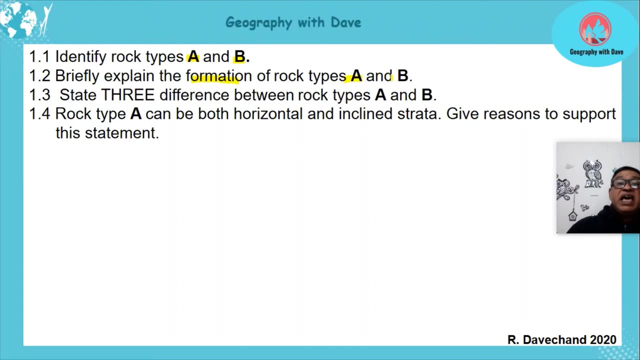 and b and you've already looked at it. if i go back, a is sedimentary and b is e. this rocks. all right, explain the formation of rock types a and b. you know sedimentary rock is a and you've already picked up from what we've discussed that erosion occurs and then sediments. 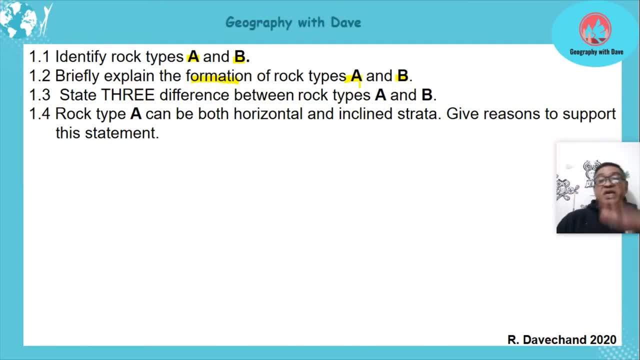 get deposited into the water at bottom and it forms a layer. as further erosion occurs, more sediments get deposited- deposited, all right, and forming another layer. the bottom layer gets compact and as more erosion occurs, further layer forms, more compact. happens, station happens, all right, and you can go through. 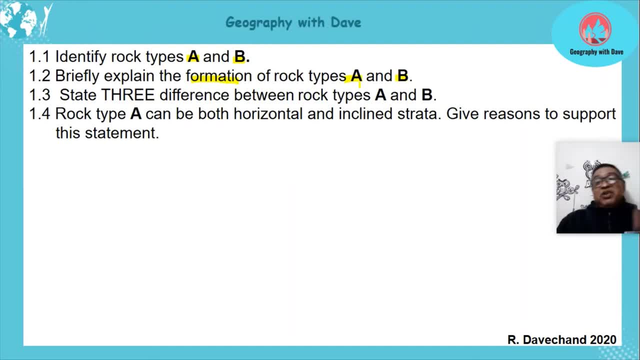 the notes again and, as this happens, whatever water is there gets forced out and we have our compact layers of rock forming your sedimentary rock. all right, very simple. you just go back, you get your notes and you work through it. all right, i can show you this very quickly again. when we 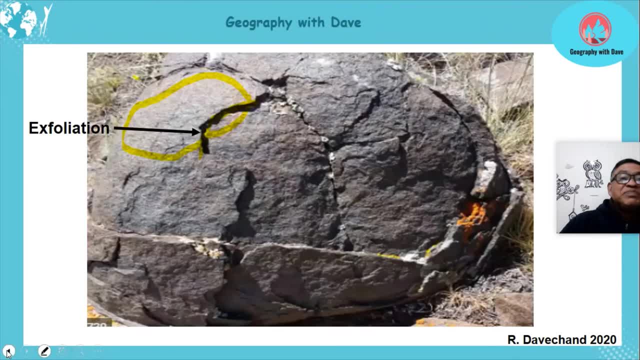 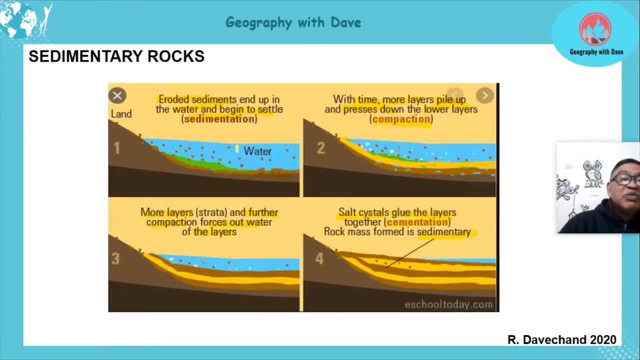 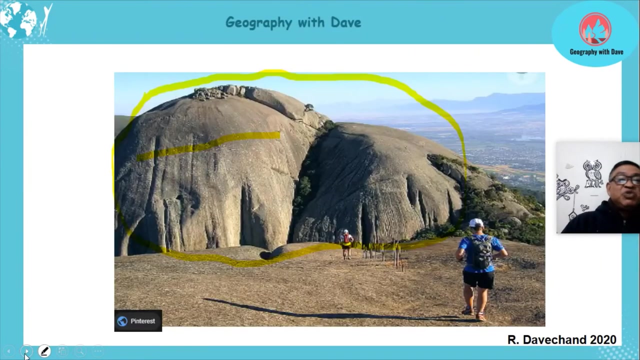 went back to those slides, all right, and there we are, all the processes of cementation, compaction. all right, and then how compaction occurs? uh, sedimentation, rather compaction, and then cementation, which forms the rock. okay, let's get back to our questions now. i just want to show you the slide. 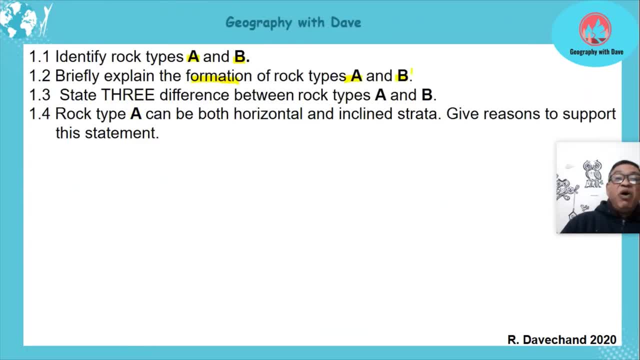 in which it was okay. then b, obviously you've learnt that it can occur below the surface, when that, so at your dike, will form a rocketed angle, all right. so various types- make沒γ道 types of rocks will form as the magma cools. but we also learn that it comes out, the magma comes. 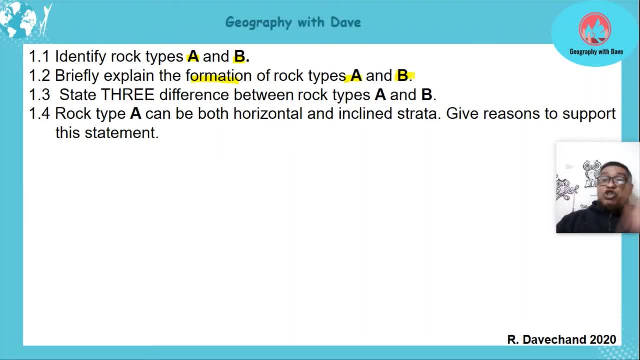 out as lava through volcanoes. it will also cool, okay, forming on the surface. with the magma, the softer rock gets eroded and therefore it gets exposed to the surface as igneous rocks. but it's all a cooling process below the surface and above the surface, all right. so let's look at that sketch. 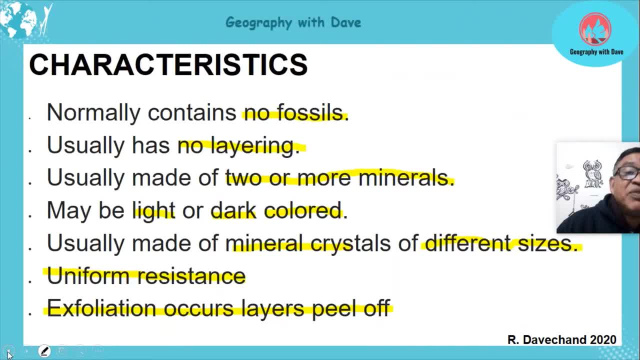 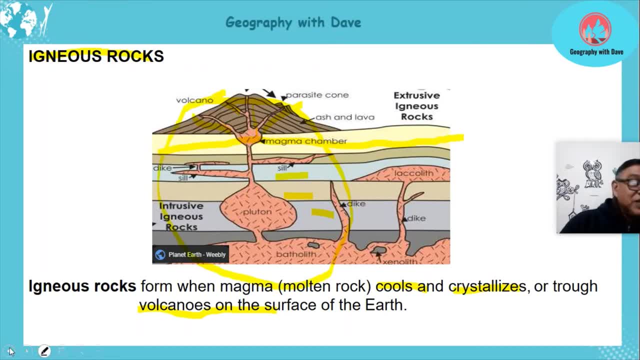 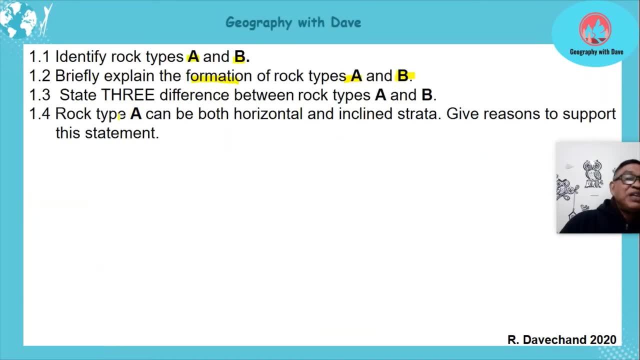 again, or that little information that i gave you. all right, can you see it here? this is the slide that we use for that with regards to the magma and the lava cooling. okay, let's go to another question. state three differences between rock type a, b. one, obviously, a has layers, b doesn't have layers. all right, b doesn't have layers, a has. 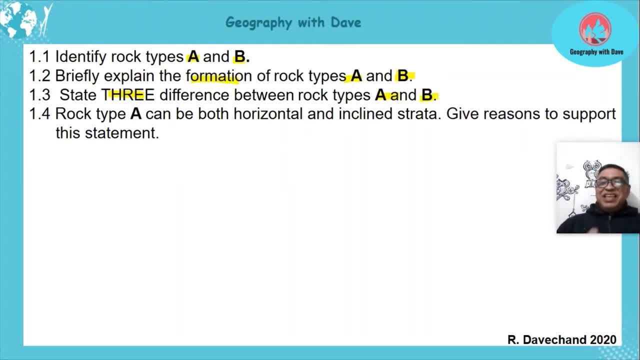 fossils. b doesn't have fossils. so a, which is your sedimentary rocks as fossils, igneous rocks- does not have fossils. sedimentary rocks, layers, igneous rocks- no, layers sedimentary rocks does not necessarily have to have you uniform resistance can be soft and hard, all right, whereas your igneous rocks have uniform. 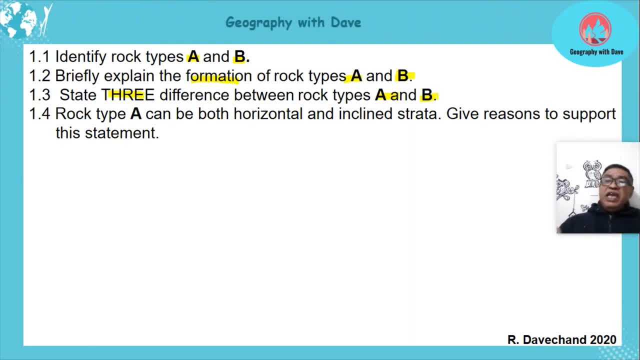 resistance. so three things: layers, no layers, fossils, no fossils and, of course, uniform resistance with igneous sedimentary not. uniform resistance, not necessarily all right. now it says a can be both horizontal and inclined strata. okay, give reasons to support the statement. so when the sedimentary rocks fall, 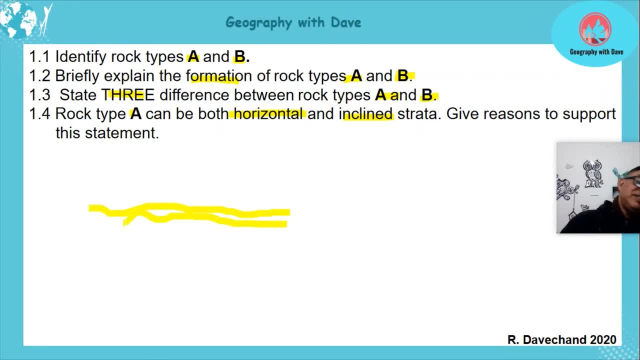 my line is not the best. i do apologize. okay, it's straight. i don't generally with the ruler, i can do it and my age is on my side. but imagine all this without no bends, but a straight line. ah, that's much better. and there's another layer. okay, that's straight. okay, let's look, focus on the straight line. 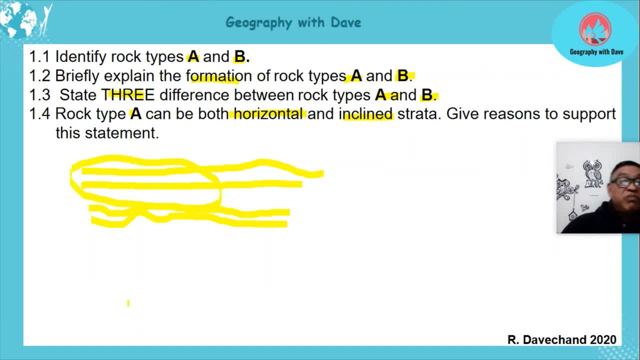 so we look at this and we have a combination there and there e the rough base here and there, right, this here and there, and there is a half base here again in the 2004 seamless disciplines. so if it's a surface here, okay of course, we just have the same. 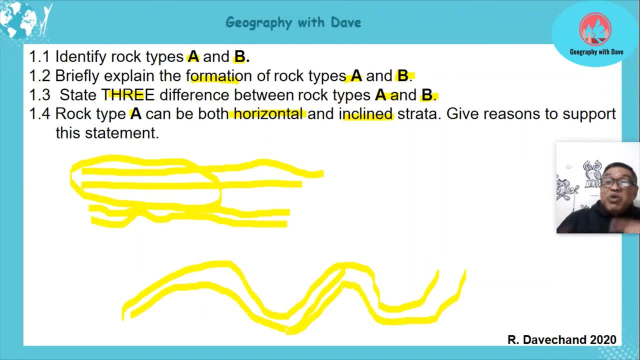 system here, of course, so that we have a visible layer in there. but now, while i'll just make Certain crystals can just pop up like that, It gives you a better understanding of how this can be horizontal and it can be inclined. all right Now. I just spoke about A, which is sedimentary.